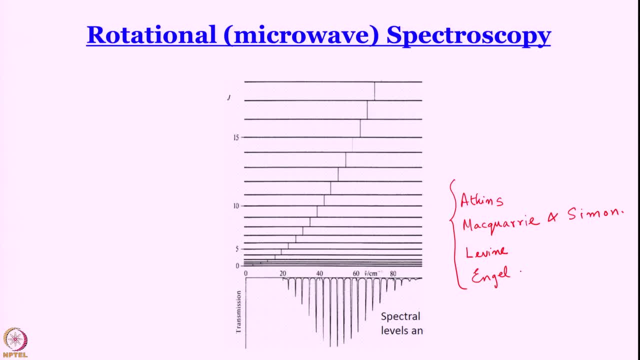 is very nice for quantum chemistry is Engel and Reed at this level. If you want to learn quantum chemistry in a little further detail, then you should study the elementary quantum chemistry book by Pilar, And there is another book by just Macquarie on quantum chemistry. 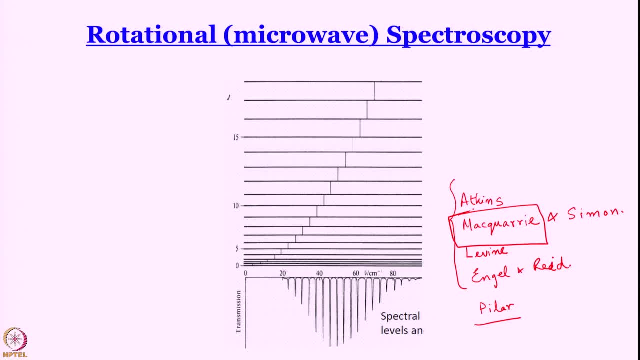 which is also excellent, And all these discussions that we are now doing on rotational vibrational spectroscopy. you would find them in all these books: Atkins, Macquarie and Simon, Levine, Engel and Reed and maybe not Pilar, And also you could study spectroscopy from the book by Banwell and 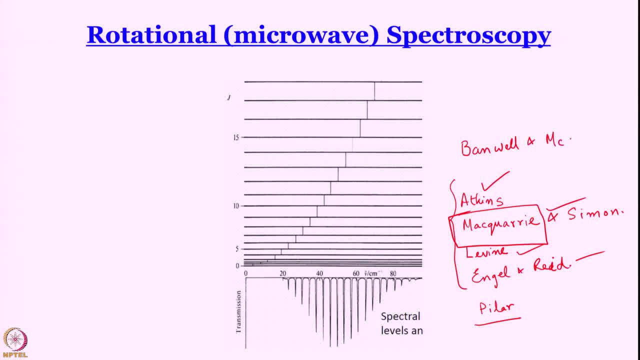 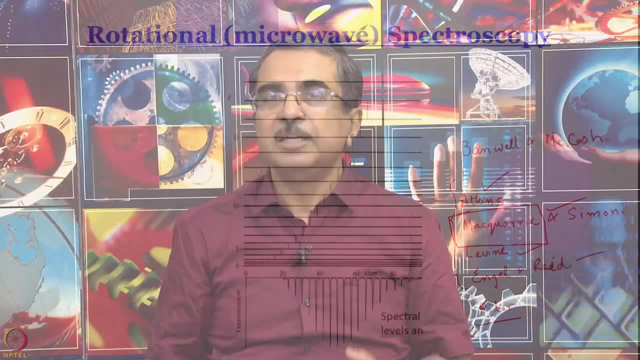 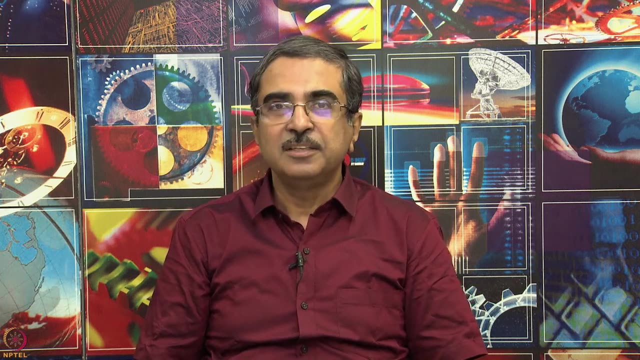 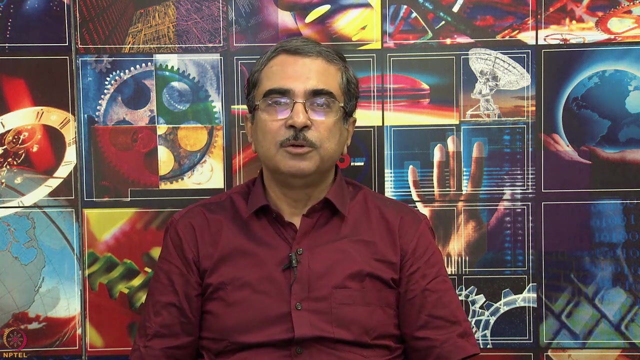 Maccash. This is the introductory book on spectroscopy that everybody studies at the beginning And then, if you are interested in spectroscopy. there are many more texts available, but we can talk about that later. That being said, let us talk about rotation of a simple diatomic molecule, HCl. Note: 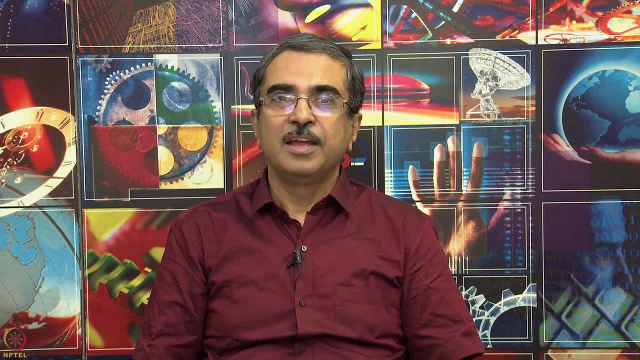 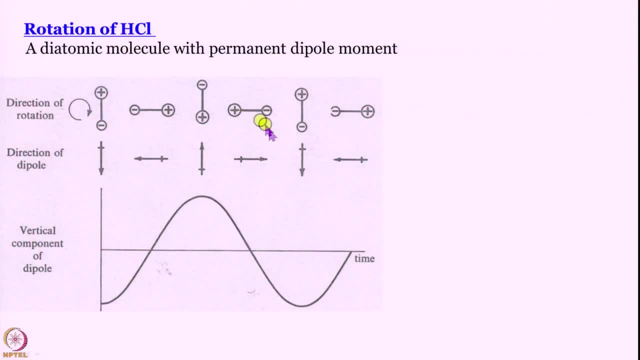 we are not talking about H2.. Why, We will see why. So what we need really is a diatomic molecule with permanent dipole moment, And this is a figure that is taken from Banwell and Maccash's book. To be very honest, I do not like this too much. 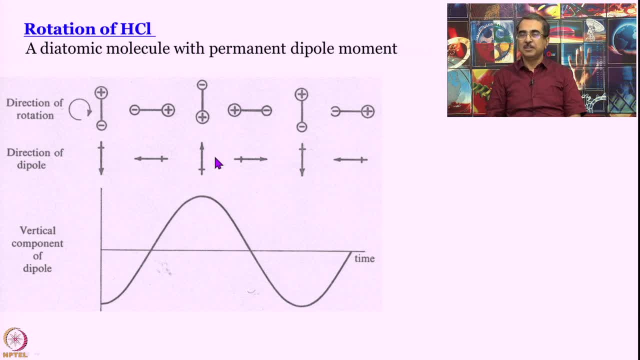 much, because it is always better to do the more rigorous treatment. Unfortunately, in this course there is no scope for it, So this should be good enough. So you will understand why it is that rotation couples with radiation by thinking like this. 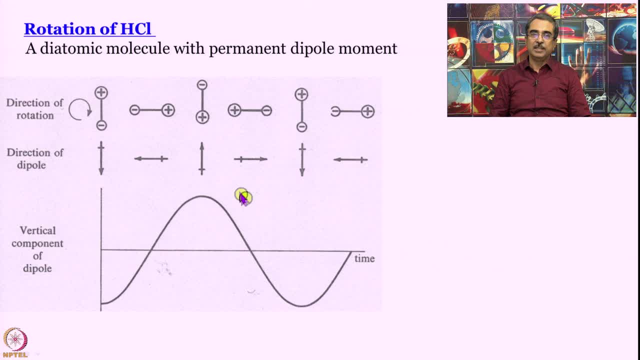 Think of this HCl molecule which has a permanent dipole moment rotating. Okay, What happens? Okay, direction of dipole keeps changing constantly. and if you plot the vertical component of dipole, then what happens? here it is negative, here it is 0, here it is positive and maximum. 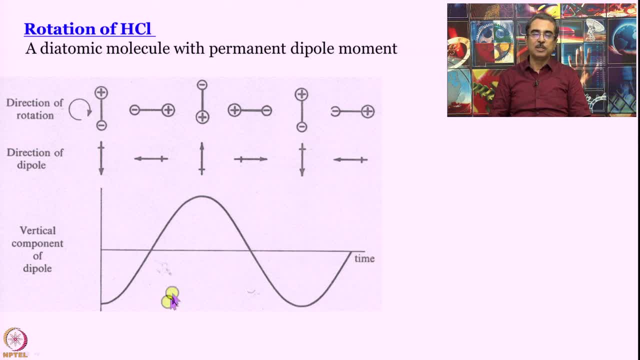 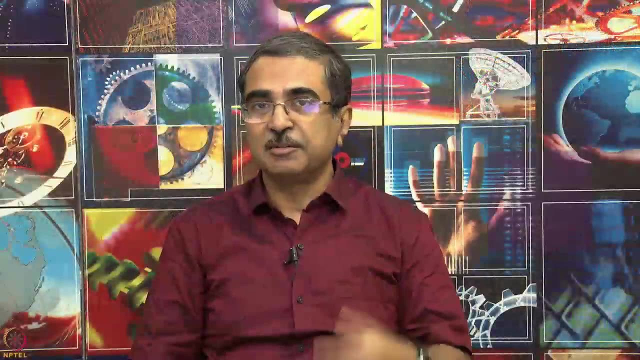 then again it is 0 negative and maximum 0 and so on and so forth. it goes on like a negative cosine wave or something like that. What is light? Light is an electromagnetic radiation, so it has electric field and magnetic field with the same frequency as a frequency of light. 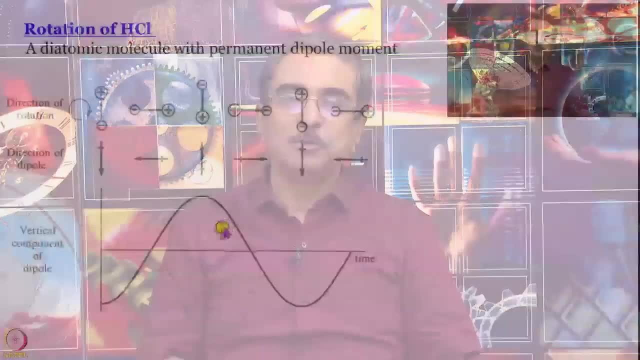 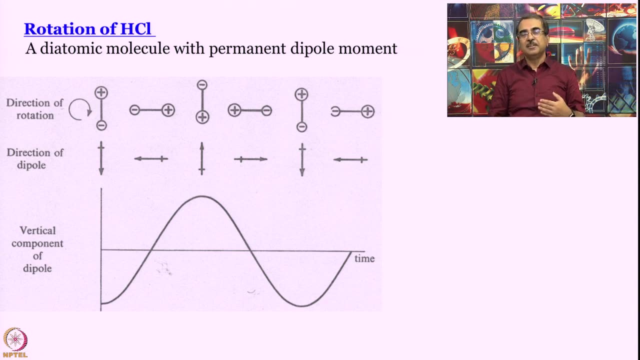 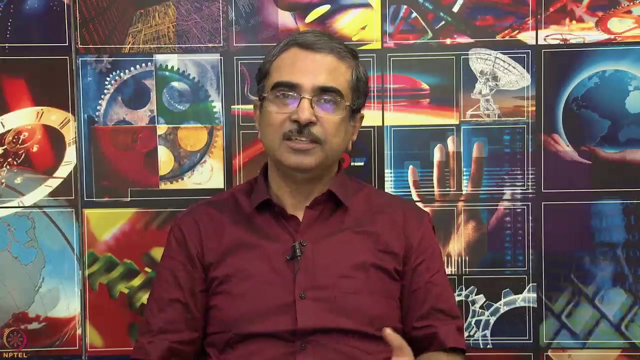 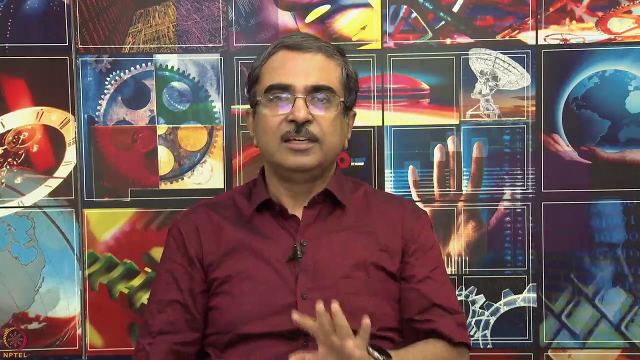 So now you can think that this oscillating electric field produced by the rotating molecule can have constructive, destructive interference with the oscillating electric field of light and that is the origin of the emission of the of spectroscopy interaction of radiation with matter. So this is a very, very rudimentary hand waving kind of phenomenon. 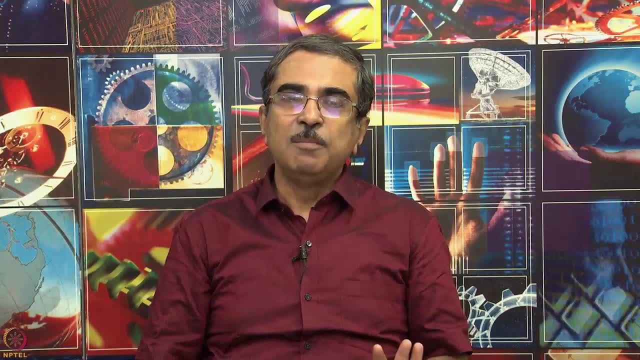 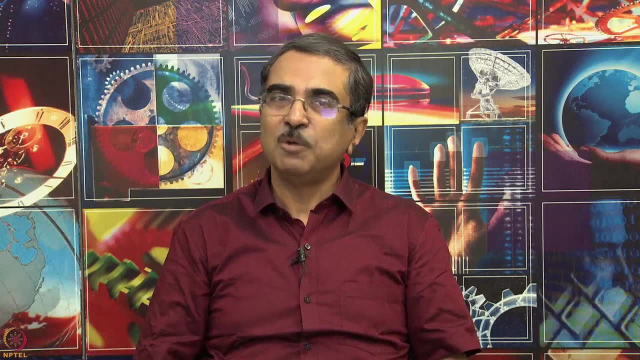 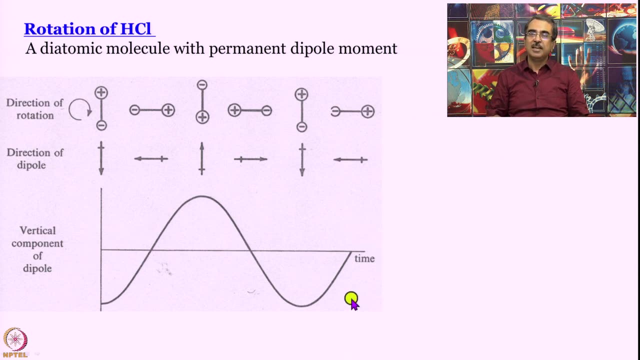 So understanding that we may develop at the moment, the important point that come out from here is that this molecule better have a permanent dipole moment in order to microwave active. this rotation is not going to produce any oscillating electric field unless that dipole moment is there in the first place, and that is why we did not say hydrogen H 2 is a non-polar. 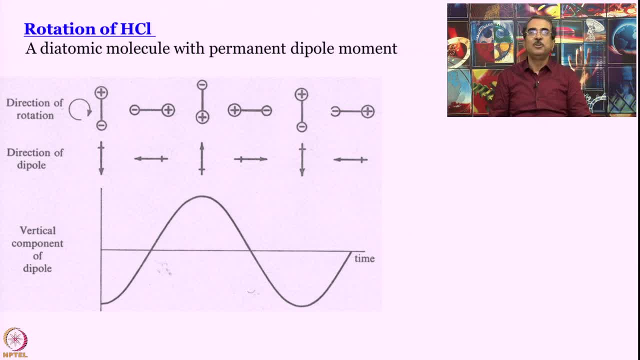 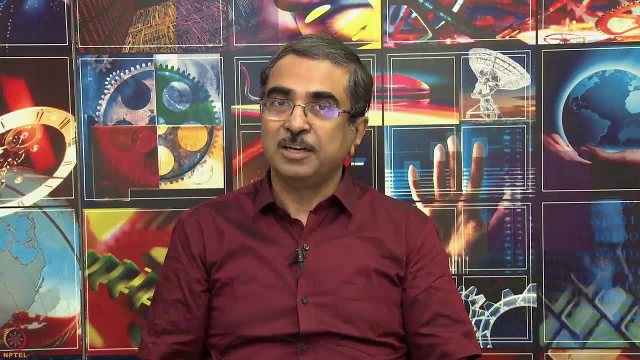 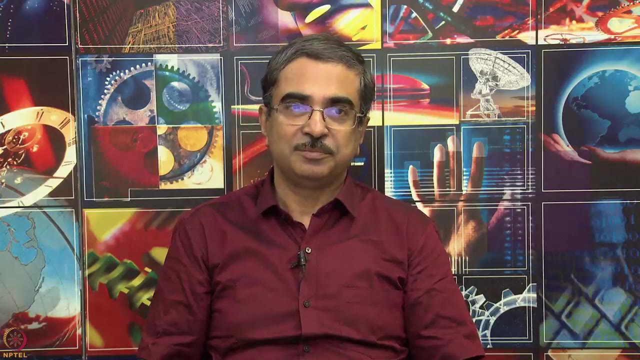 molecule. So, no matter how much H 2 might rotate, it is not going to interact with microwave microwave. Does that mean that we cannot study rotational levels of H 2? No, it does not mean that we can find it using something called rotational Raman spectroscopy, Unfortunately. 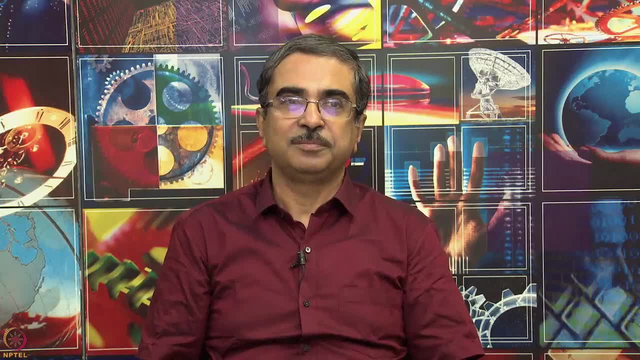 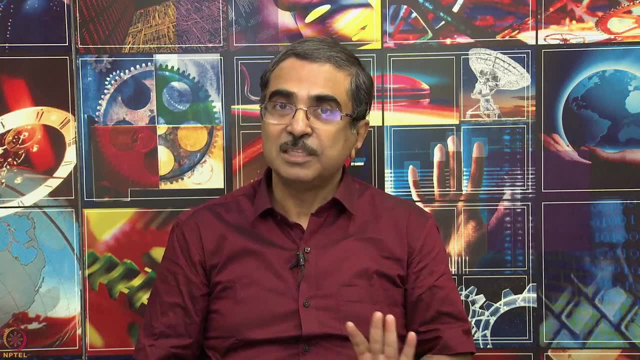 in this course. we are not going to get into Raman spectroscopy Now. so that is the first condition. it requires a permanent dipole moment, and that immediately opens up several applications, at least one of which is perhaps very well known to each other. 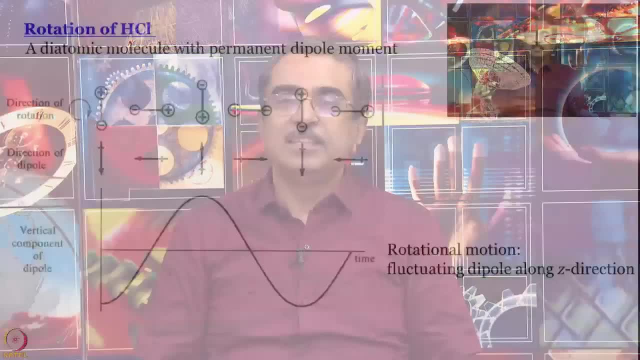 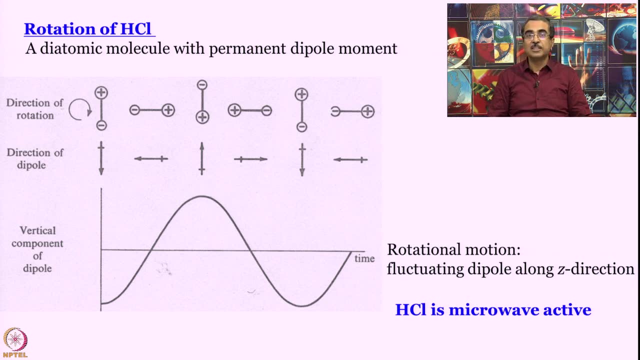 happens in our household. So this is the essential condition. and HCl is microwave active. water is also microwave active because water can also be approximated as a dipole. it is a polar molecule, So even rotation of water can give you microwave activity, and that is an important point, remember. 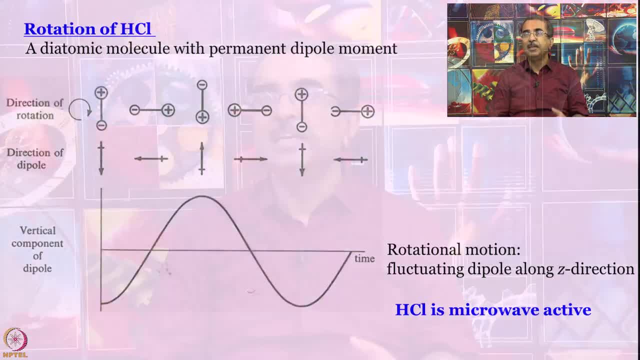 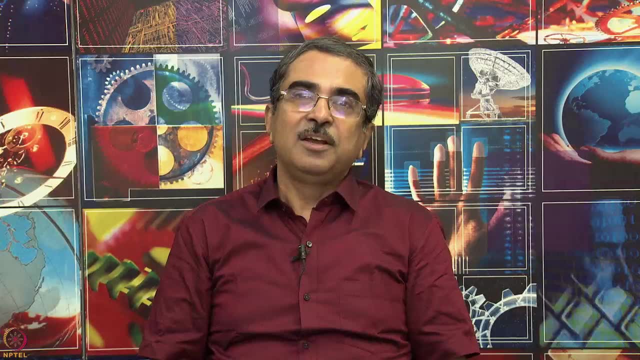 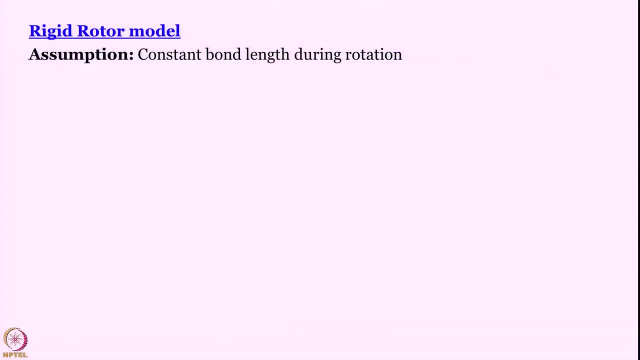 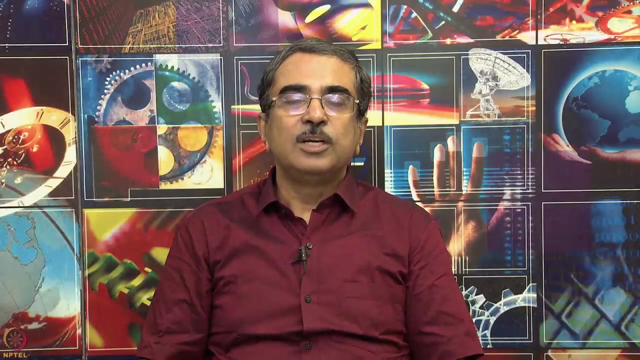 in our discussion To build a quantum mechanical description. what we use commonly is a rigid rotor model. The assumption here is that during rotation the bond length does not change. Once again, it is an application of Born-Oppenheimer approximation. So let us say this is: 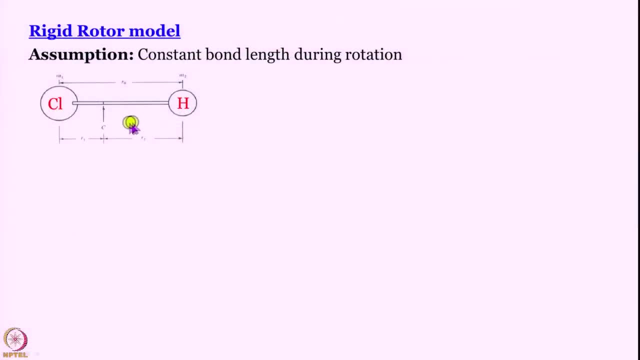 the molecule we are talking about, HCl. this is the bond length separation between the nuclei, and we have considering the molecule to be stationary. I mean we are considering the bond length to be same. that means the molecule is not vibrating or anything during rotation. 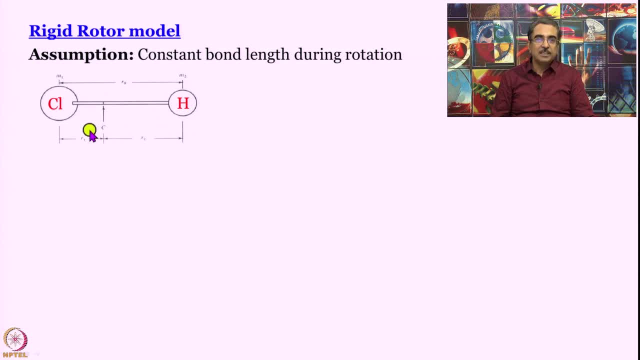 So now see this fine print that you see. here are the C, here is the center of mass and of course, Cl is much bulkier atom than hydrogen, So the center of mass will be displaced towards Cl. R0 is the bond length. this R1, R2 are there, and this is a little problematic model to use. to start, 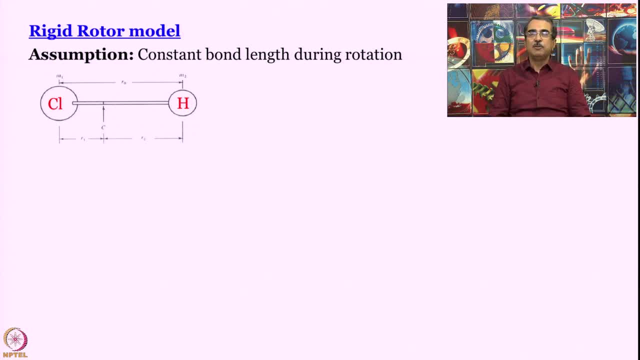 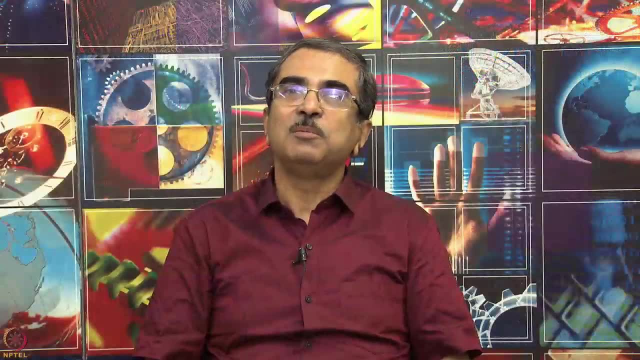 with, because there are two bodies. If you try to write the equation, you will have too many terms. So common approach of something like this, again coming from classical mechanics, is that you reduce this two body problem to a one body problem. This is what the one body problem looks like. So 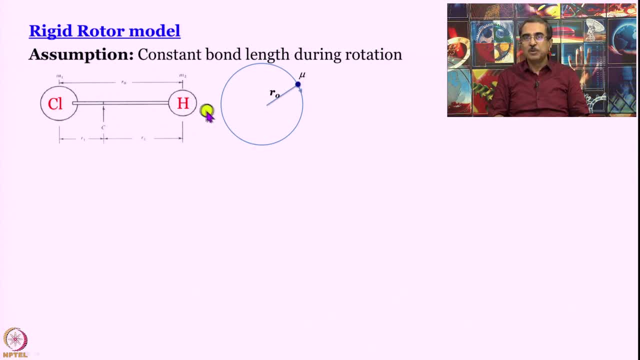 the reduced mass. I hope you know what reduced mass is. we have discussed it earlier: 1 by mu, equal to 1 by H, 1 by mH plus 1 by mCl, where mH and mCl are the masses of hydrogen atom. 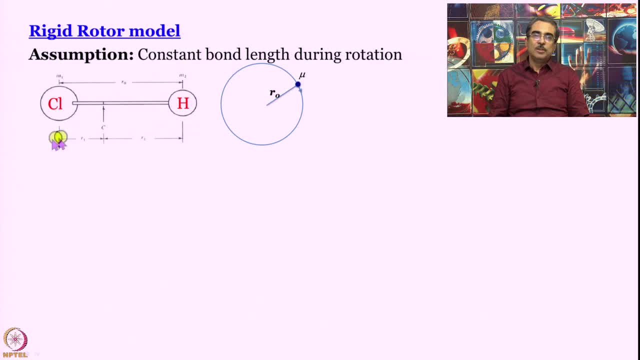 and chlorine atom respectively. So this problem is reduced with a little bit of manipulation, which I believe we have studied in rotational dynamics in class 11 physics. This problem is reduced to a single mass, a single atom, a single particle with mass. 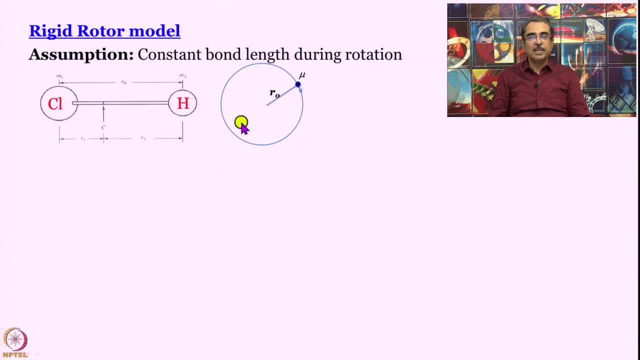 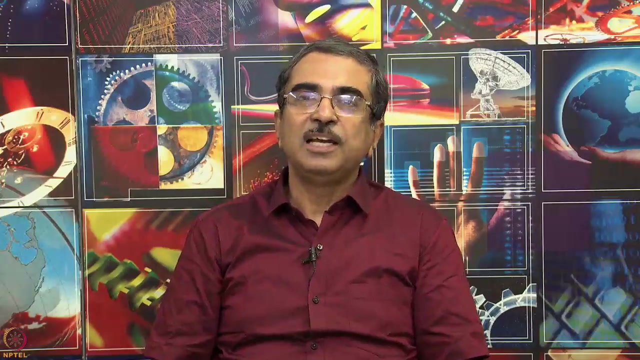 equal to reduced mass mu rotating around. a. note: this now massless, chargeless center. Separation between the center and this mass is R0, the bond length. Now a couple of comments here. In HCl, what is mu going to be like? Is it going to be like the? 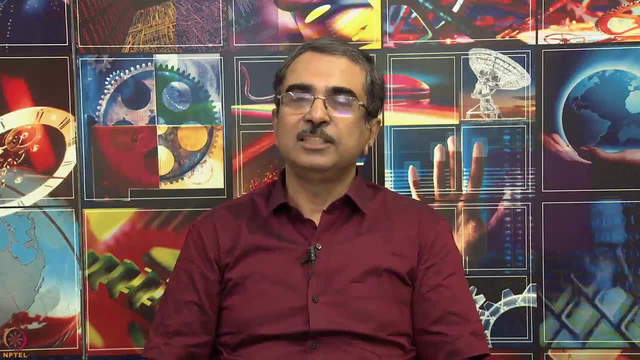 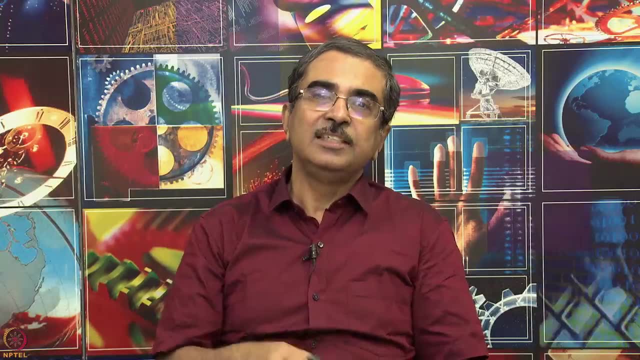 mass of hydrogen or is it going to be like the mass of chlorine? The answer is it is going to be like the mass of the hydrogen. So this is the mass of the hydrogen. So it is almost like hydrogen is going around chlorine and chlorine is stationary. It is just. 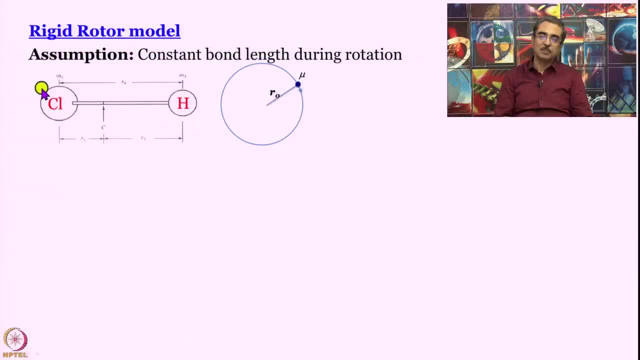 that, since we have used reduced mass, we do not need to consider the mass of chlorine anymore, So the center can be considered to be massless completely. Have we encountered this situation earlier? Actually, we have, is not it? When we set up Schrodinger equation for hydrogen, we had written the Hamiltonian theta phi. 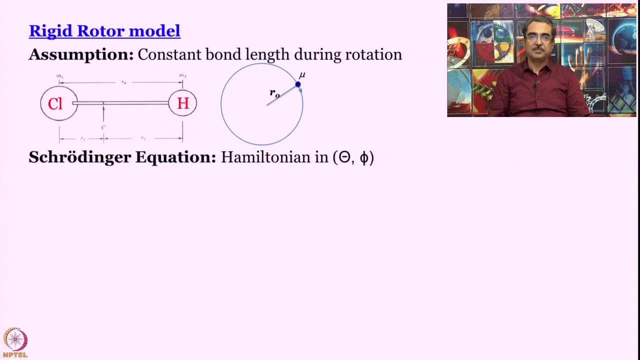 this was actually the inherent assumption. So what we will do now is that we will try to see what the solutions are In fact, since the Schrodinger equation is similar to that of hydrogen atom angular part, the wave functions are also the same as in hydrogen atom spherical harmonics. 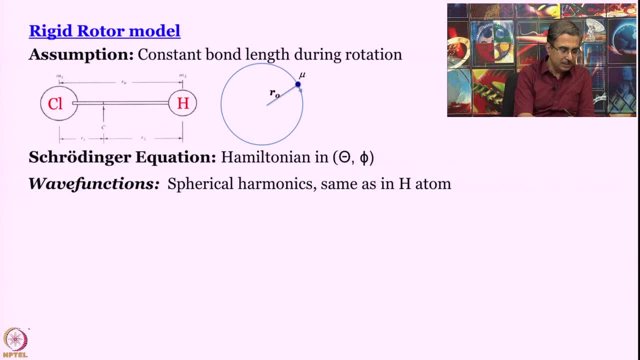 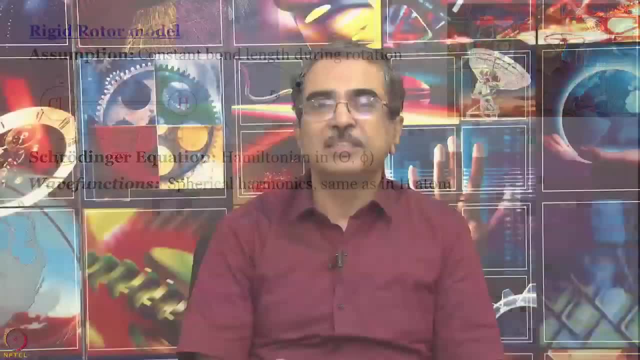 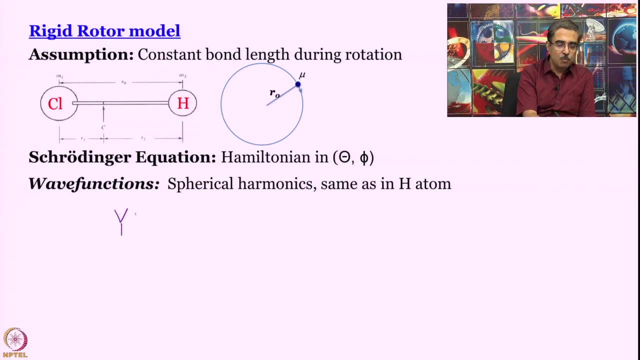 Since we know that the wave functions are spherical harmonics, same as hydrogen atom, we can try to work with them. What do we know about the spherical harmonics of hydrogen atom? We know that in spherical harmonics- we have written them as y- which have functions of theta and phi. 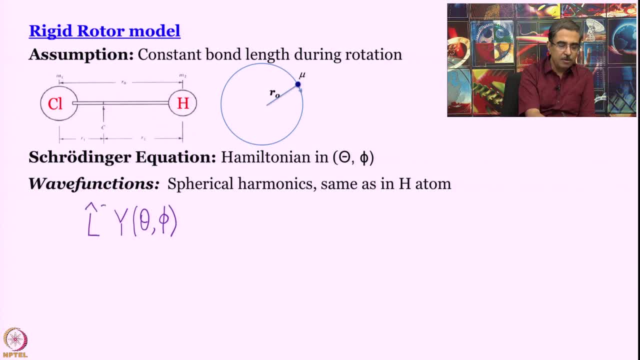 They are eigen functions of the l square operator with eigen value of l into l plus 1 multiplied by h, by 2 pi h cross, not really H square divided by 4 pi square. Here the difference with hydrogen atom is that this r is constant, So we can. 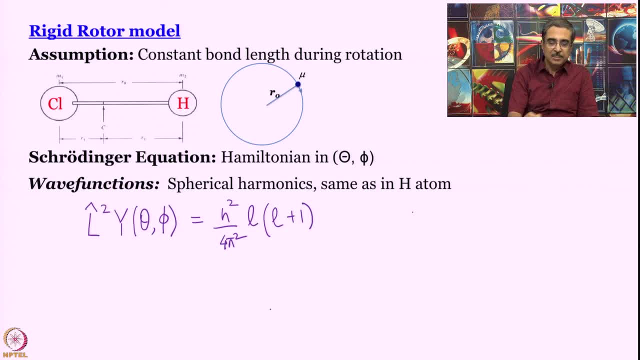 try to find out what is the rotation energy here? How Remember the relationship between kinetic energy and angular momentum? It is L? square by 2i, is not it? So if I take this L square operator and divide by 2i, what is i? i equal to mu r 0 square. Then what do? 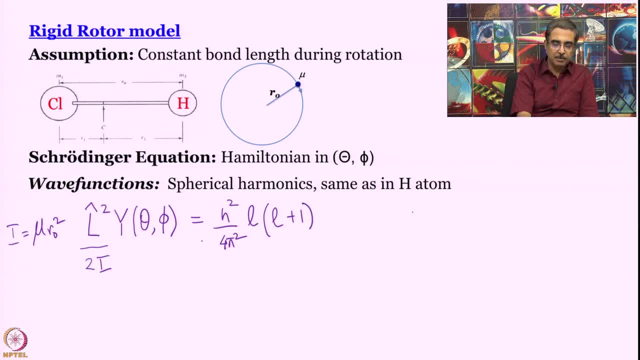 I get. I get h square by 4, pi square multiplied by 2i, multiplied by L, into L plus 1.. We will make only one change here: We will not write L. When you talk about rigid rotor, it is conventional to write J as the quantum number. 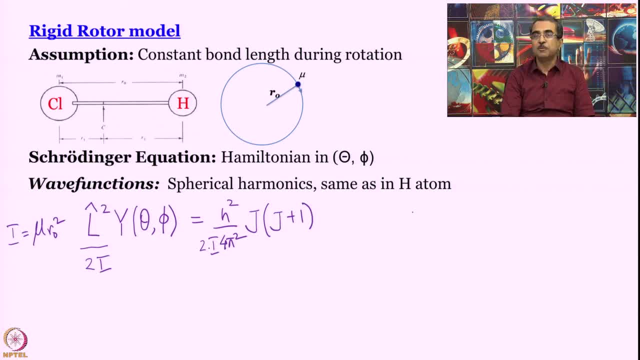 Instead of L, What is J? J is the rotational quantum number Very, very similar, or well, for all practical purposes, same as the azimuthal quantum number in hydrogen atom. So let us write it a little better. This turns out to be h square divided by 8, pi square i into. 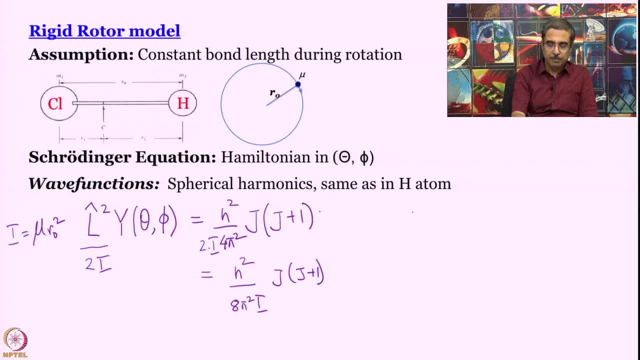 J into J plus 1.. I forgot to write this y theta phi here Multiplied by y theta phi. What does this mean? We said earlier that this here is the kinetic energy operator, So I can write it as maybe t theta phi operating on y of theta. 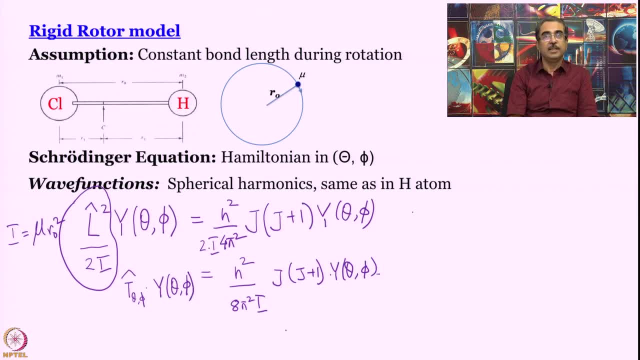 and phi. So this is what we get: an eigenvalue equation. This here is the eigenvalue. So this is kinetic energy. It is as simple as that. Is there a potential energy for rigid rotor? No, because we have defined it as a one body problem, as a mass going around a massless, chargeless center. 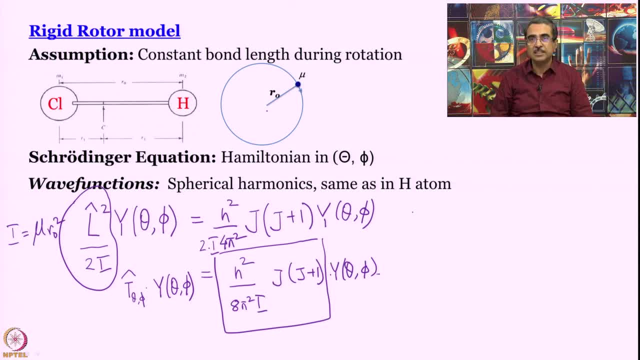 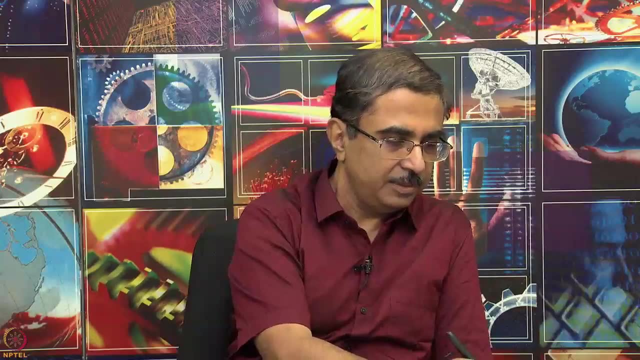 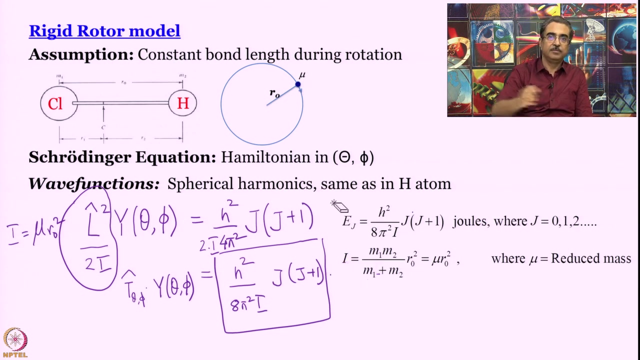 So in that case, if the center does not have any mass or charge, then there is no question of potential energy that can arise. The energy of a rigid rotor is purely kinetic energy, So it is now. So this is what the expression is: E, J equal to h square by 8, pi square, i, J into J plus. 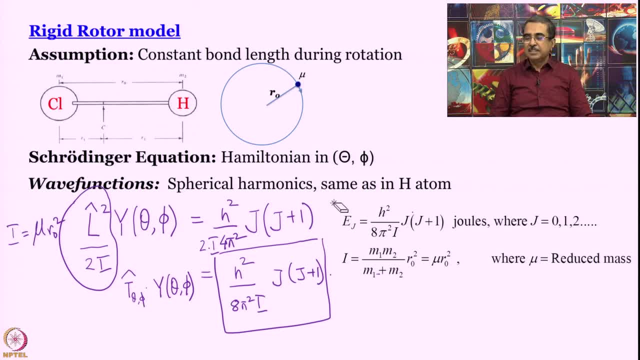 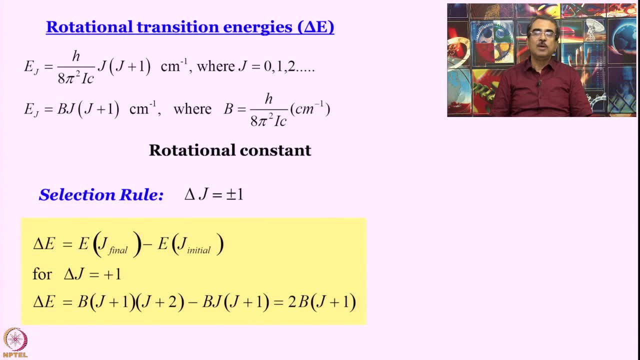 1 in Joule. Now, generally it is conventional to not work in Joules. When we talk about microwave spectroscopy, we like to work in wave numbers. So how do I write the energy in wave numbers like this: This is the energy h by h dij: This is the energy of micro spectroscopy. 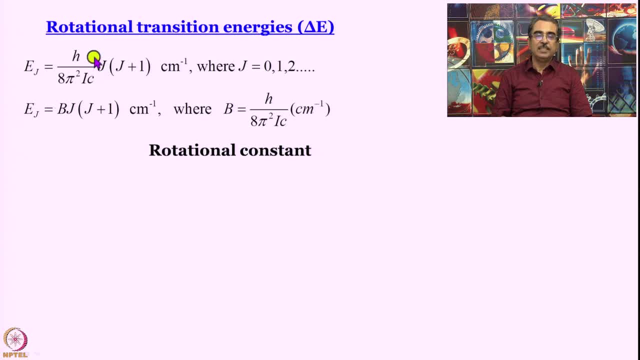 So when we take haggle spectroscopy, we will get this energy. As what should the поб Earth as much as possible to minute weight, great energy activity: 8 pi square i c. How did we get it? How did we get this in the first place? 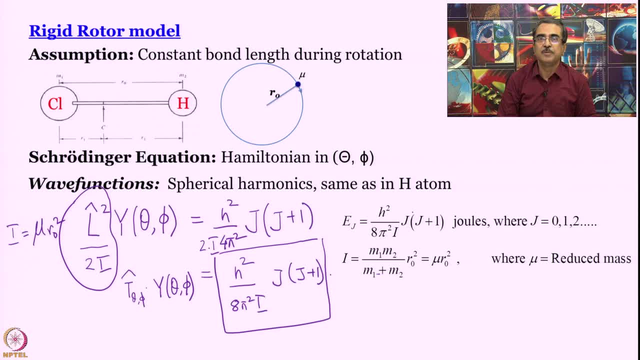 How do we get energy in centimeter inverse? Well, this thing has to be divided by h- c. So just bring in an h c here. What happens? This h and this h goes and we have a c left in the denominator. That is what gives us the expression. 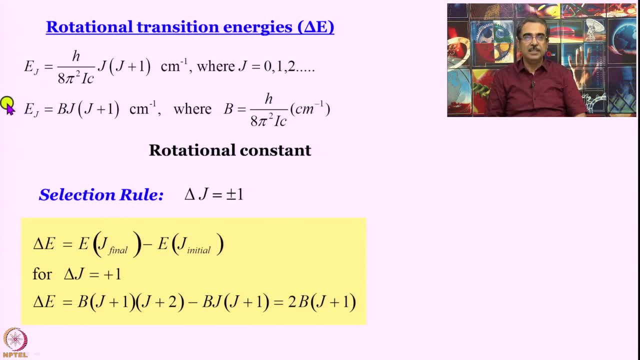 Actually it is conventional to write epsilon j here. Here we have written e, ej equal to h by 8 pi square i, c multiplied by j into j plus 1 centimeter inverse where j is 0,, 1,, 2, exactly like your subsidiary quantum number of hydrogen atom. 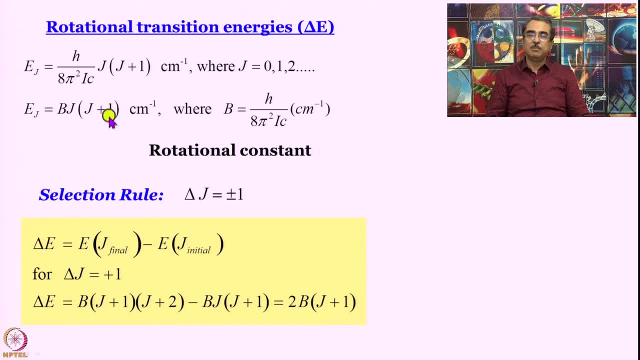 So in short, it is written: ej equal to b into j, into j plus 1 centimeter inverse, where b, h by 8 pi square i c. this here is the rotational constant in centimeter inverse. There is a selection rule. I told you earlier that not all transitions take place, So 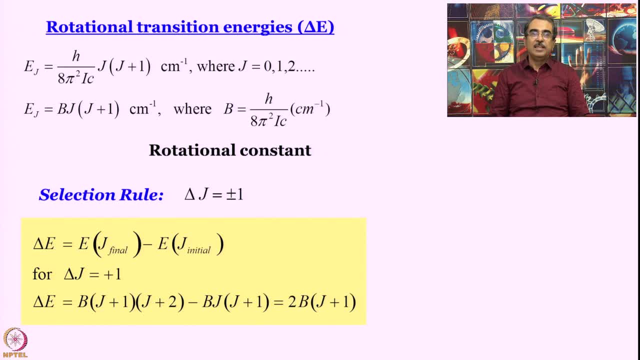 selection rule. without going into the derivation here, is delta j equal to plus minus 1.. So what would be delta e for delta j equal to plus 1? You just substitute the values and work out b. what is the energy for the jth level? b, j, j plus 1. to know the energy of the j plus 1th level: 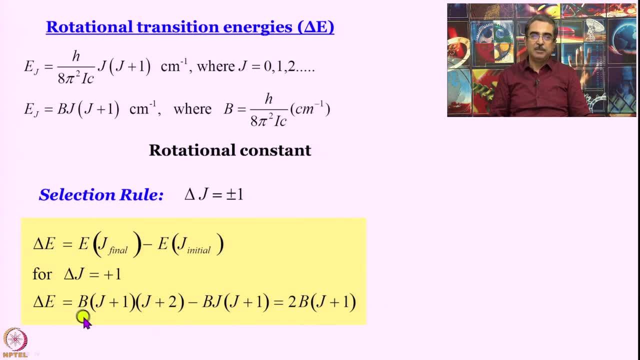 I just have to write j plus 1 in place of j, So it becomes b into j plus 1 into j plus 2. subtract this from here. you get 2 b into j plus 1.. So what does it mean? It means that it means: 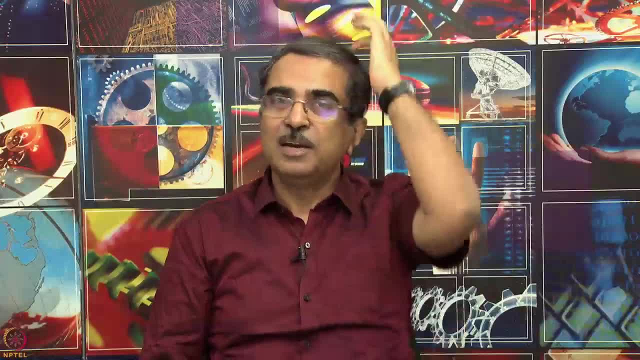 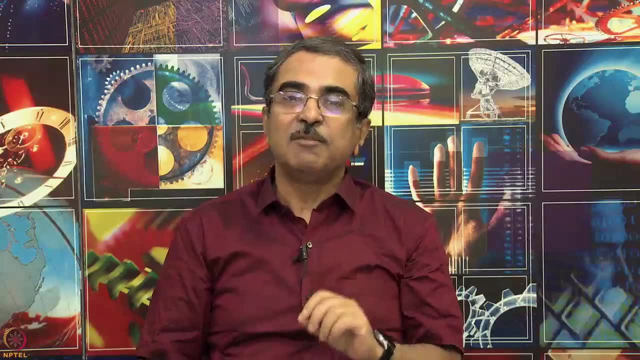 two things. first of all, the energy levels are separated by 2 b into j plus 1. we are going to show you the diagram. Secondly, your rotational spectral lines will also occur at 2 b into j plus 1. of course, we get line spectra. 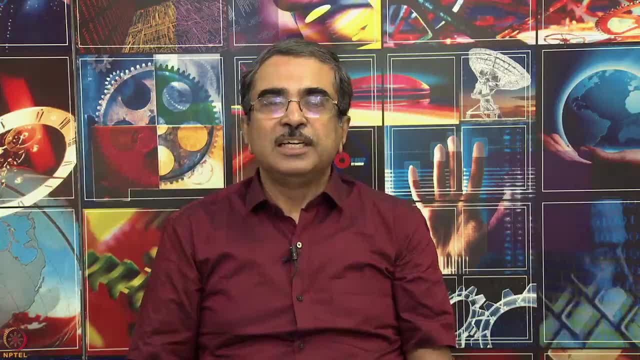 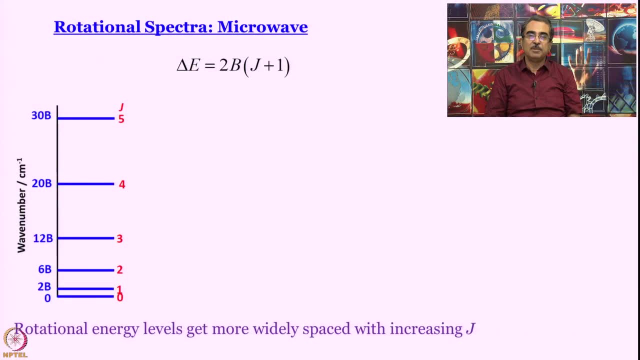 So where? what do the spectra look like? First, let us draw this energy level ladder that we talked about here. it is it b, j, j plus 1.. So if it is b into j, into j plus 1, when j equal to 0, it is 0. 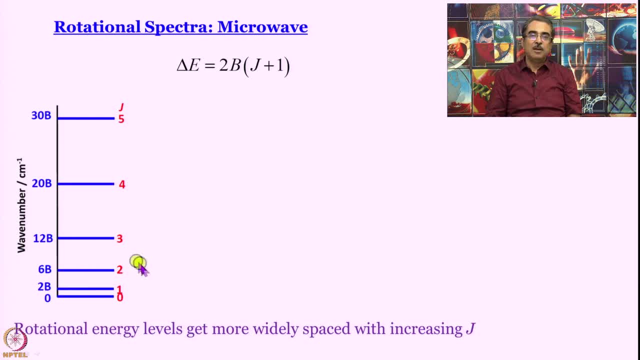 and j equal to 1, b into j, into j plus 1 is 2 b. when b equal to 2, then what happens? j is 2, j plus 1 is 3, 2 into 3 is 6, 6 b, so on and so forth. So, as you see, the energy gaps keep on increasing. 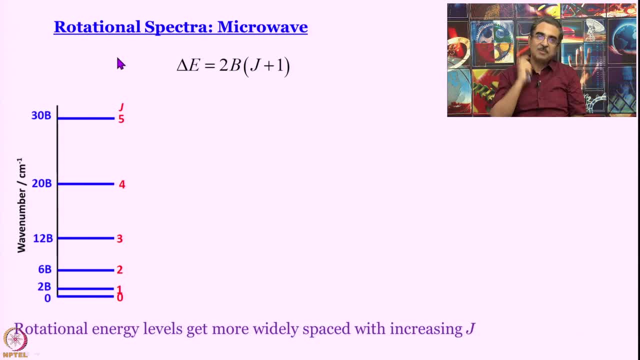 as you go higher up the ladder. does that ring a bell? does that remind you of particle in a box? Now, what about the spectrum? Where will the lines be? The first line will be for transition between 0 to 1. that will be at 2 b. second line will be for transition between 1 and. 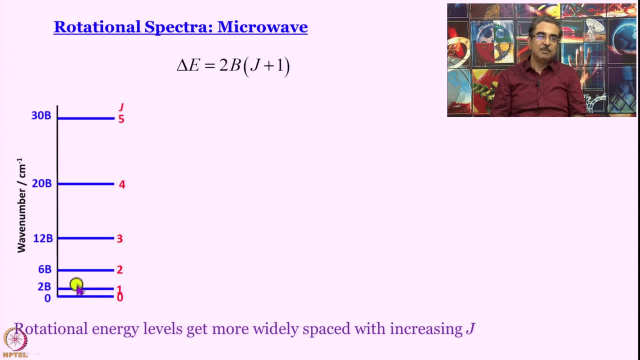 2, that is 6 b minus 2 b, 4 b. third line might be between 12 b for transition from 6 b to 12 b, n equal to j, equal to 2 to j, equal to 3 level, that is 6 b, and so on and so forth. 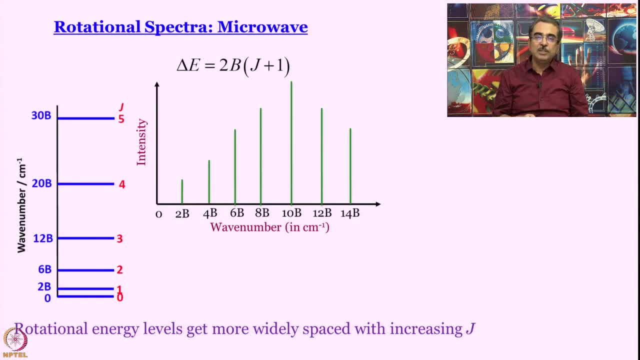 So this is what the spectra look like. you get an equispaced spectra where spacing is 2 b in each case. spacing between two successive lines is 2 b of what uses that? well, since they are equally spaced, and from the spacing you can find out what the b is. you can actually 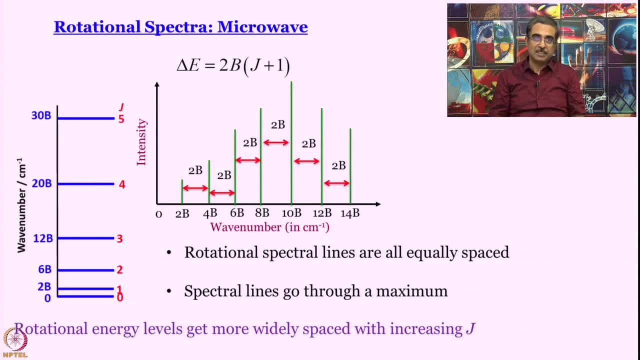 determine the bond length, can you? they do go through a maximum. why they go for maximum, we will come to that, But even before that let me at least mention that. is not it clear that from the spacing of the spectral lines we should be able to find out what the- if you know, the reduced mass? 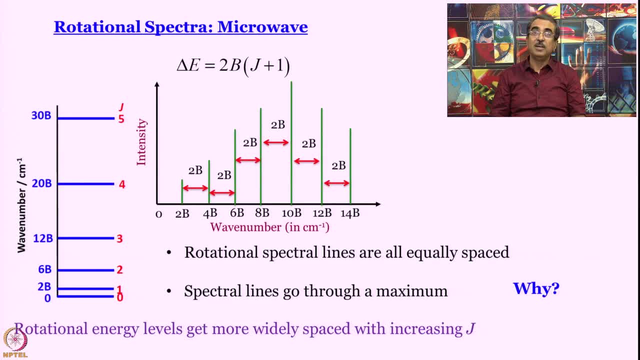 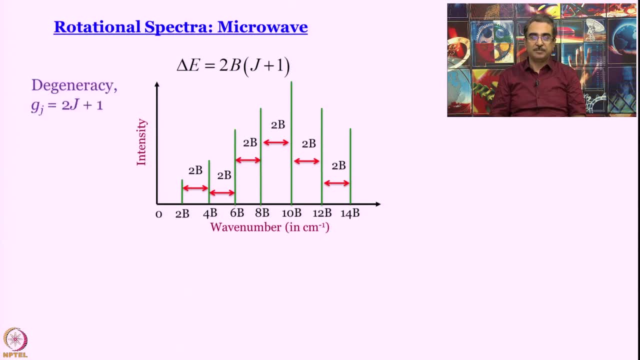 which there are easier ways of Finding. you can find out what the bond length is. we are going to come back to that. before that, let us address this question: why is it that the spectrum goes through a maximum? this is why, see, each rotational level actually is 2 j plus 1 fold degenerate. remember this, remember those l. 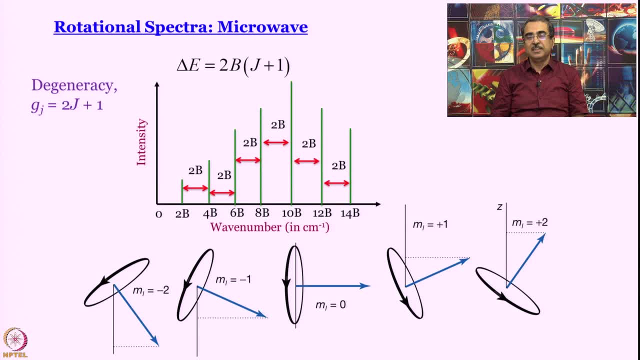 levels, all of them, where 2 l plus 1 fold degenerate. and, as we said, we just substitute small l by capital j here. So you get this angular momenta pointing in specific different orientations, and how many such directions are allowed depends very much on which j you are working with. So g j equal to 2 j plus 1. here we have given. 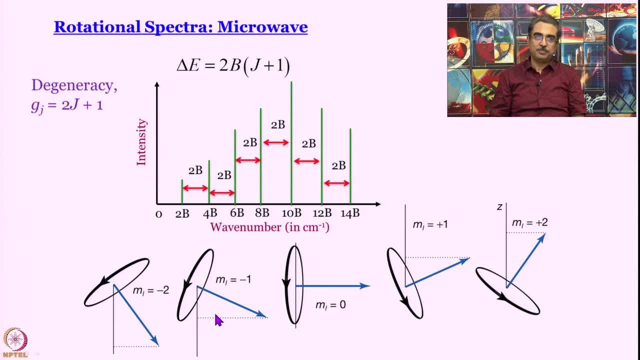 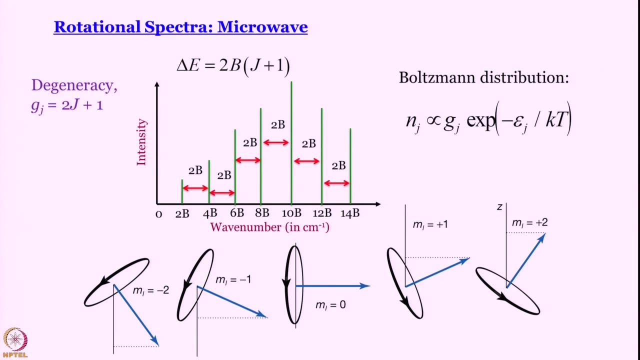 you an example of j equal to 2.. So degeneracy is there? what happens to degeneracy then? as you go higher up the level, degeneracy increases. And what is Boltzmann distribution? It is g, j multiplied e to the power, minus epsilon j by kT. So epsilon goes up with j, So e to the power. 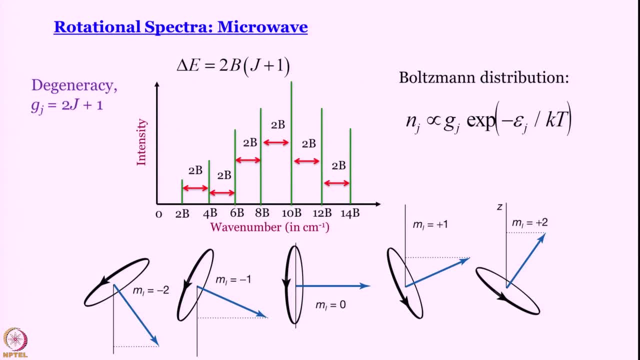 minus epsilon j. epsilon- here is just that. e that we wrote earlier. e to the power minus epsilon j by kT will go down with increase in j, So that is a decreasing function. Degeneracy is basically a straight line with j, So multiply a straight line with positive slope. 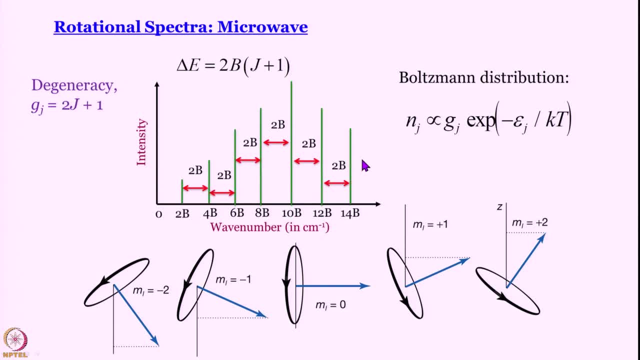 by a decreasing function. what do you get? You get something that goes to a maximum. This is why rotational spectra go through a maximum. Homework for you is: find out an expression for j in which population is maximum. I will just discuss how to do it. This is how you do it Essentially: you take dnj, dj equal to 0. 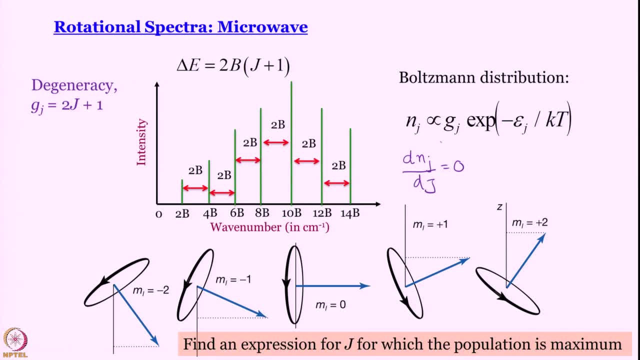 At maximum, the first derivative will be equal to 0.. So take a derivative of this. What is this? 2j plus 1 multiplied by e to the power minus, here I will write j minus ej. divided by kT, This is equal to 0.. 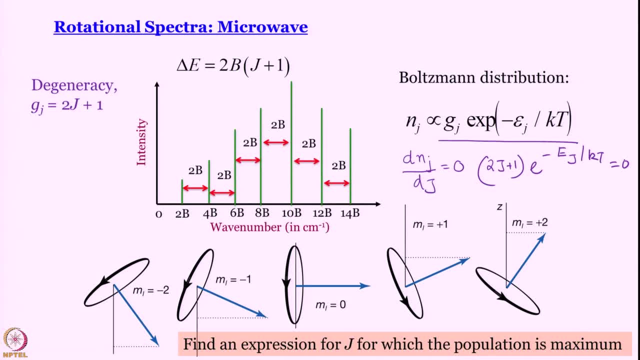 So what are the solutions? Is this right what I have written? Not really, So this ddj of this is equal to 0.. Now you can do this differentiation: find out what you will get, And what you will get always is. you will get an expression with two terms. 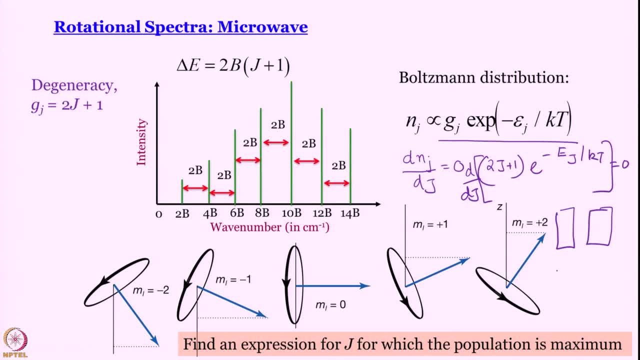 I will not tell you what the two terms are. But you substitute, you will get j equal to maybe 10.23.. So what does that mean? It means that, see, here we are using calculus which inherently requires continuous variation. We do not have continuous variation here, We actually have discretization. 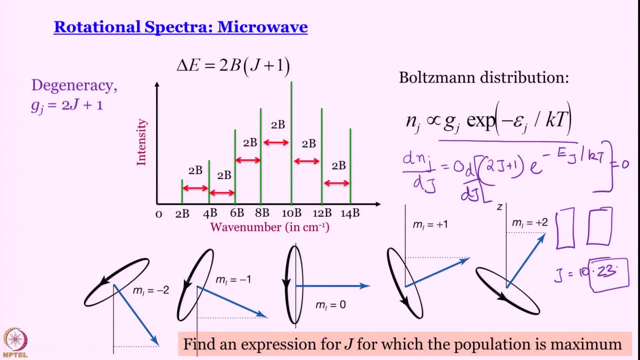 So that is why this 0.23 or whatever it is it comes. You have to neglect this point. just work with the whole number that comes out. You can take the nearest integer that is going to be the value of j where the population is going to be maximum. Please do it yourself if you have. 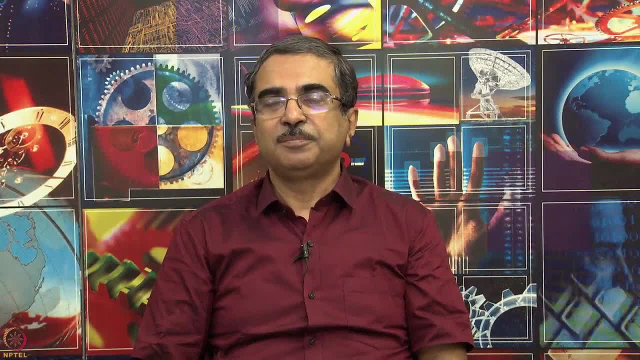 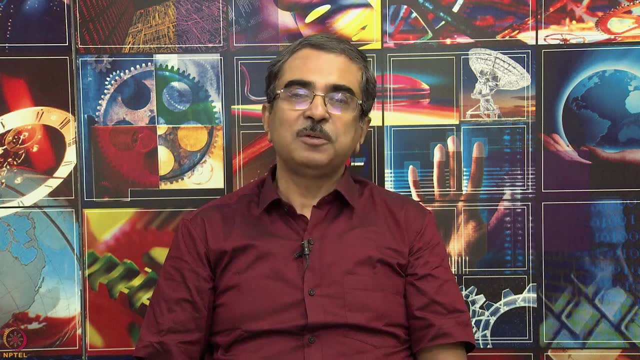 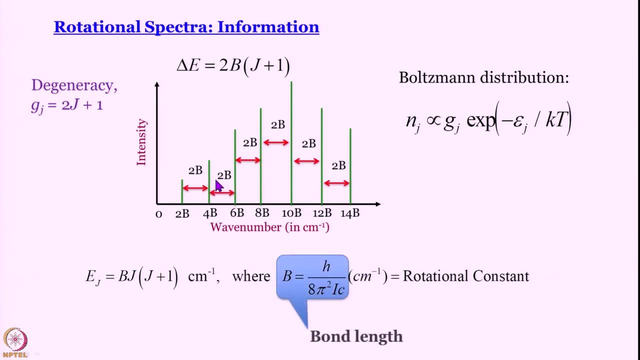 any difficulty. it is worked out in Atkins book as well as Manuel and McCash's book. So what is the information that we find? I have played a spoilsport and we have already told you that when you look at this spectrum from the spacing, you know what 2b is that is going to. 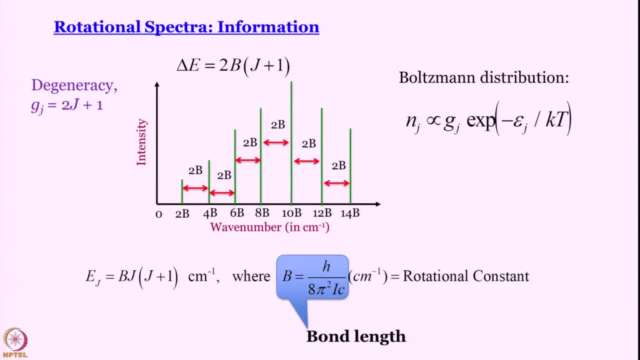 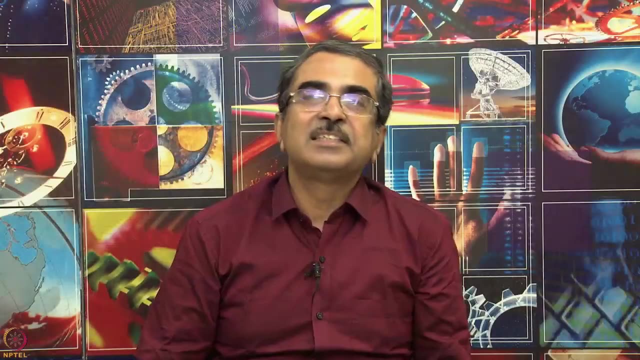 give you bond length, because i, after all, is mu r 0 square. If you know mu from here, you find b is a very elegant, easy method of finding bond length. what kind of molecules? only those molecules that are dipolar H2 cannot be done this way. you need Raman spectroscopy Now. in the last lecture we 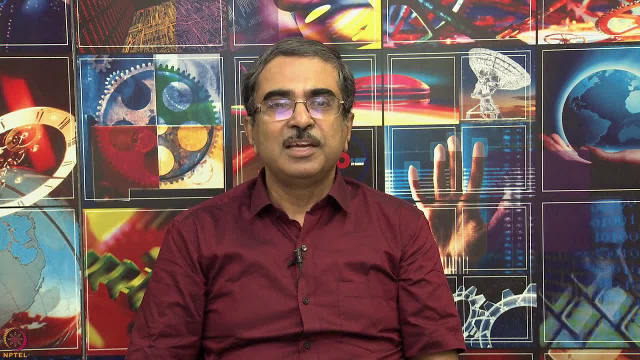 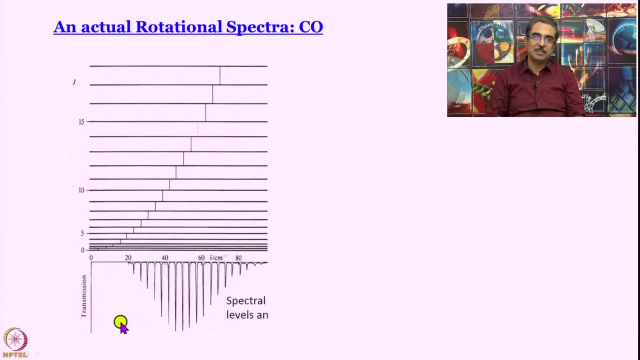 talked about what Planck had said about experiment. so you cannot close it without showing you an actual spectrum. This here is a spectrum of carbon monoxide, rotational spectrum. You can see more or less equispaced, and here they have plotted transmission. that is why it is. 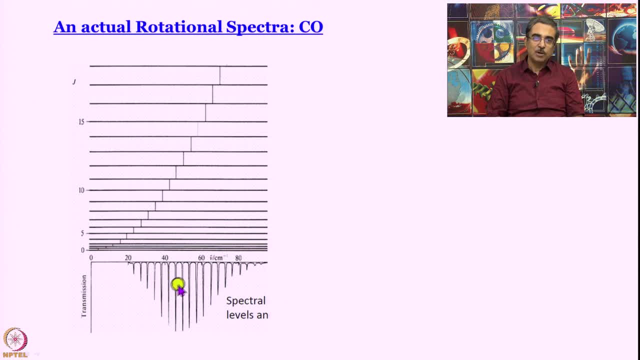 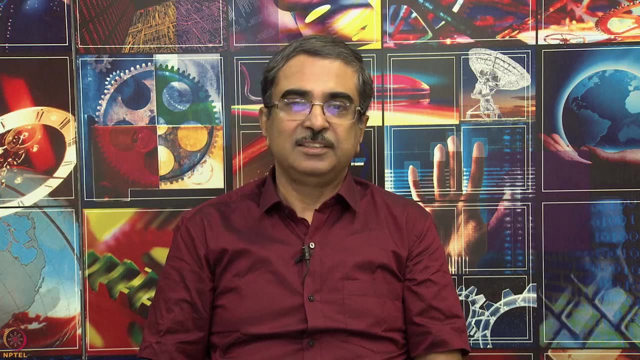 negative going. But you can understand that if you work out the spacing here between any 2 lines, you can. knowing the masses of carbon and oxygen, should be able to work out the bond length. So this is one of the applications, but there are others. Second application: is that commonplace? 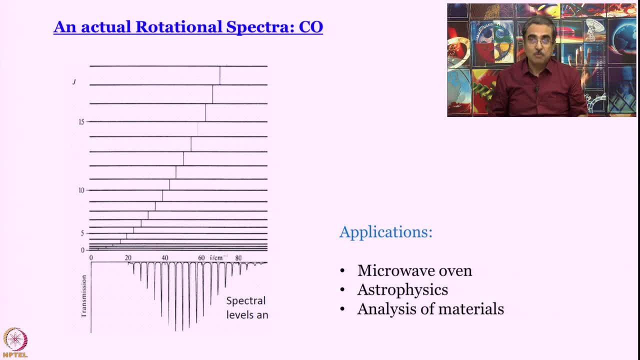 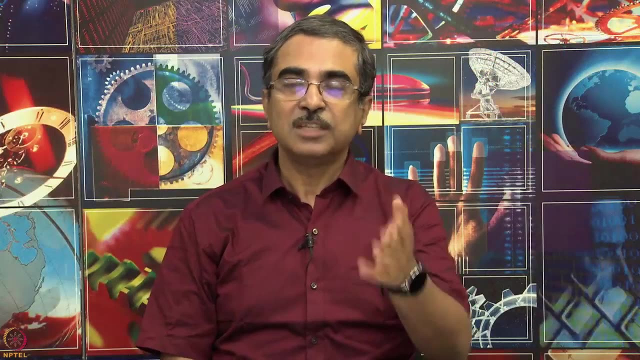 thing that we are talking about microwave oven. Why is it that food gets hot if you place it in a microwave oven? Why is it that food gets hot when you place it inside a microwave oven? Because, unless you are somebody who eats nails and stones- 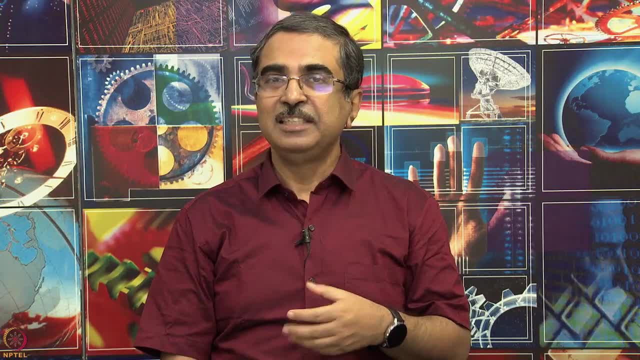 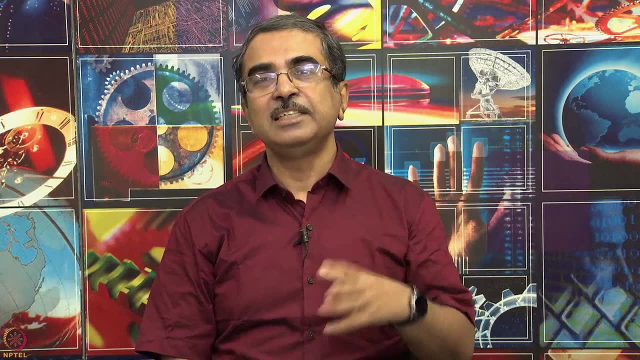 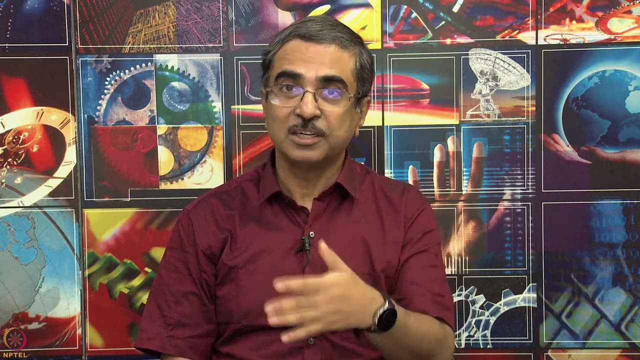 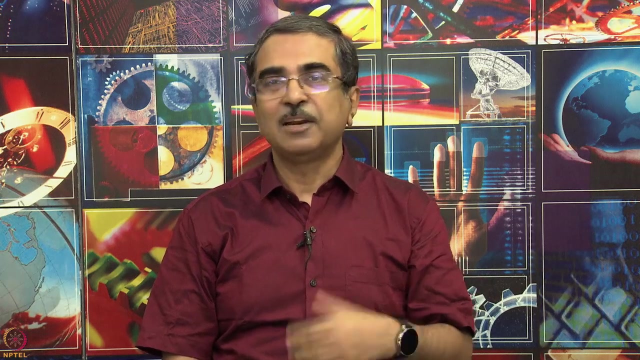 for dinner. most of the food that we eat is 70% water. So when you place it in microwave oven, microwave of the frequency that is broadly absorbed by water is incident on your food and it actually goes through other glass and oil container. So all this water inside your food starts rotating. it gets energized, but they cannot. 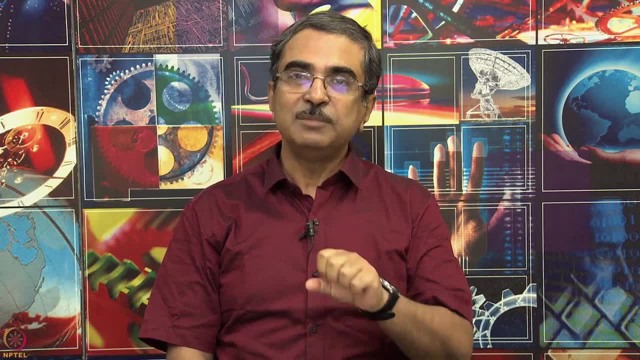 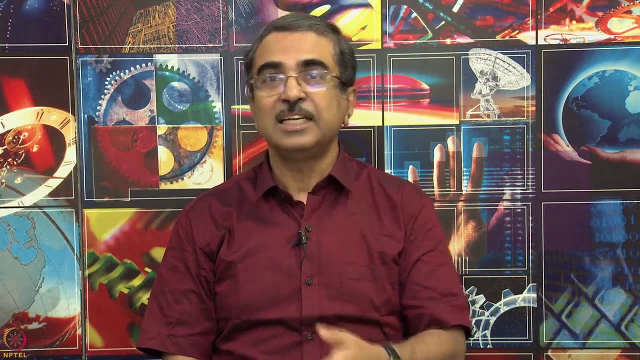 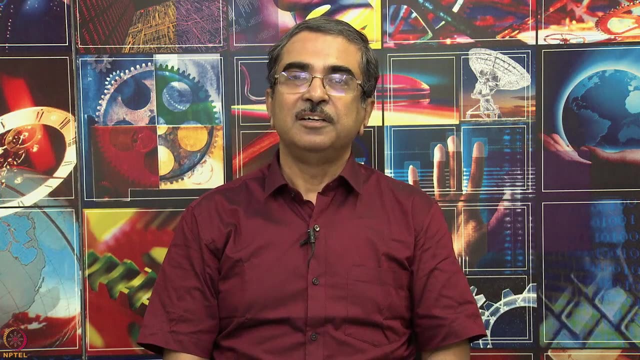 keep rotating. always they have to stop. When they come to stop, that is because of dielectric friction and that is when this rotational energy they are acquired is given to the surroundings. that is the food in the form of heat, and since there is 70 percent water, it is sort of like fire. 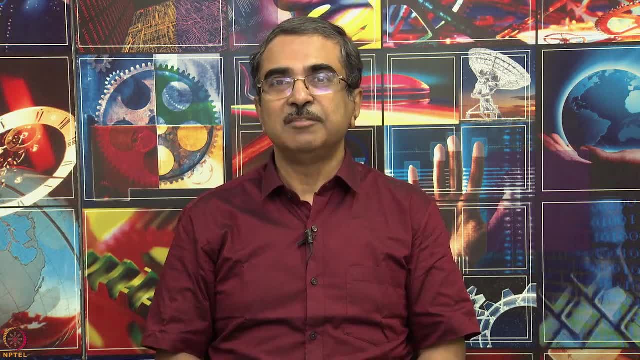 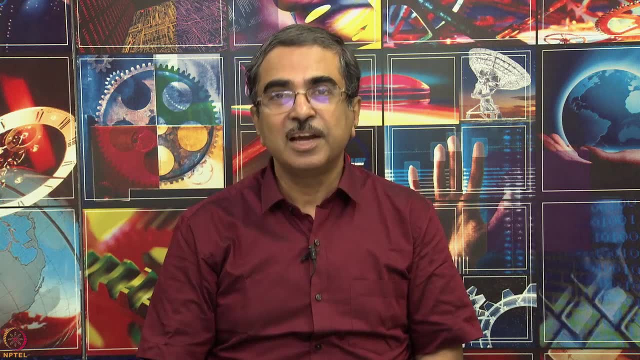 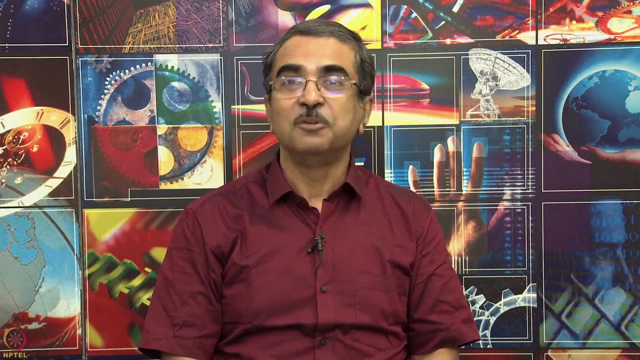 within. That is why microwave is a very efficient way of heating up food or cooking it. Mind this, you cannot fry anything in a microwave because to fry you need to go beyond 100 degree centigrade. you need to get your oil heated. oil is non-polar, it is never going to heat up. you can cook. 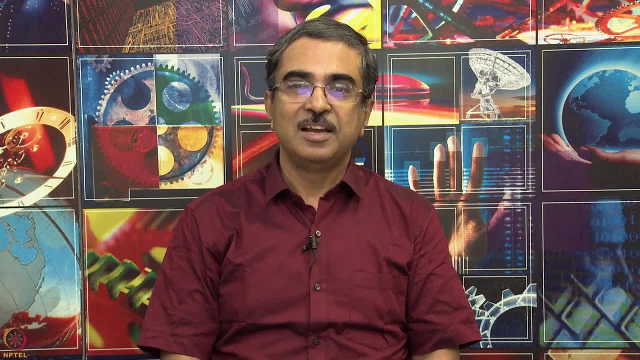 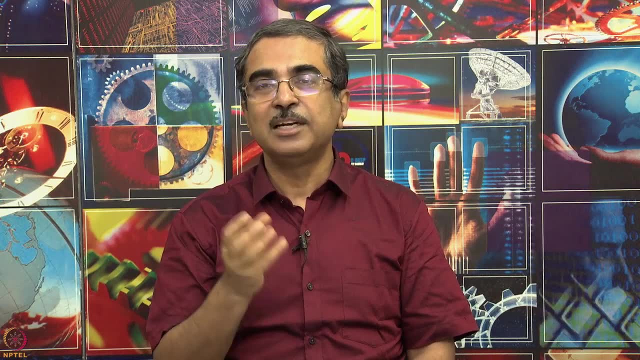 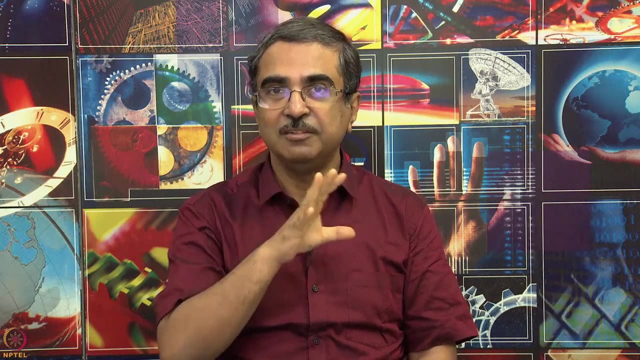 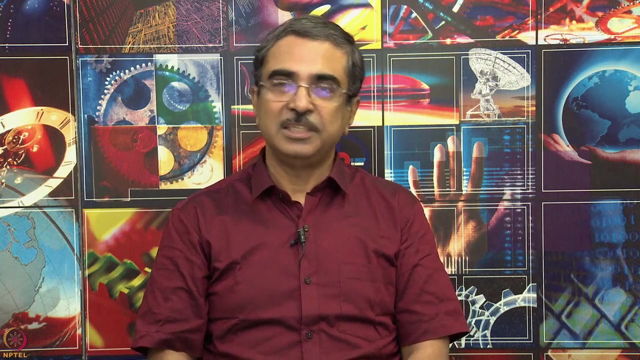 you cannot fry in microwave. Astrophysics is another area where microwave spectroscopy has a lot of application. look at microwave radiation and from there you can tell which molecule is there in that, but the environment of that particular star, or even planet, I think, And it is used for things like fault analysis in analysis of materials. So microwave spectroscopy